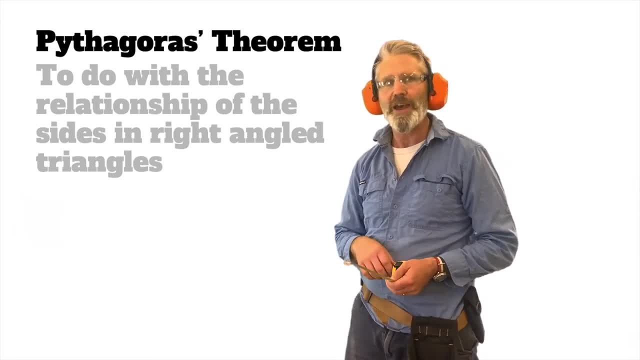 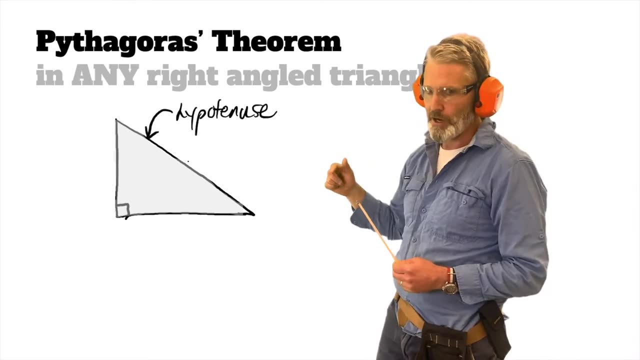 happens in all right-angled triangles And in actual fact, it says that in any right-angled triangle, the hypotenuse, which is the long side opposite the right angle, the hypotenuse squared, will be equal to one of the shorter. 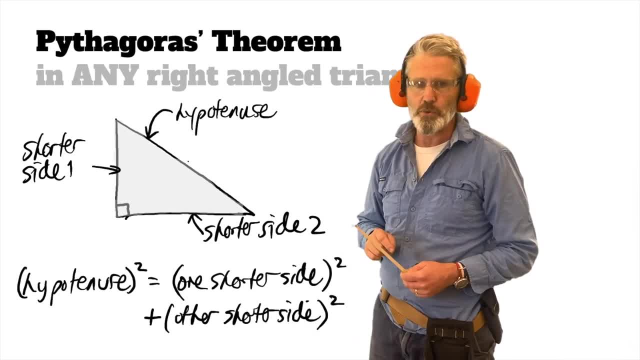 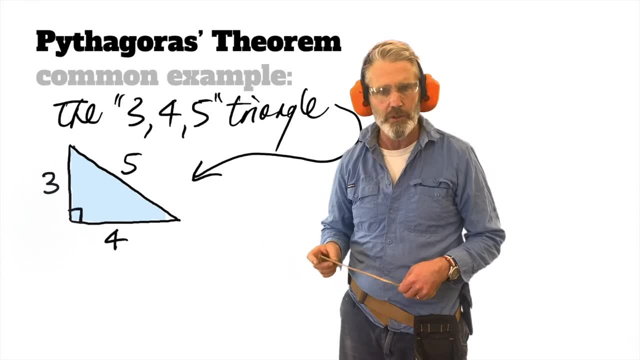 sides squared plus the other shorter side squared. Now there's a really famous ratio of the three numbers that work with this. That's the 3-4-5 triangle, and that works because 5 squared is 25.. 5 squared is 25.. 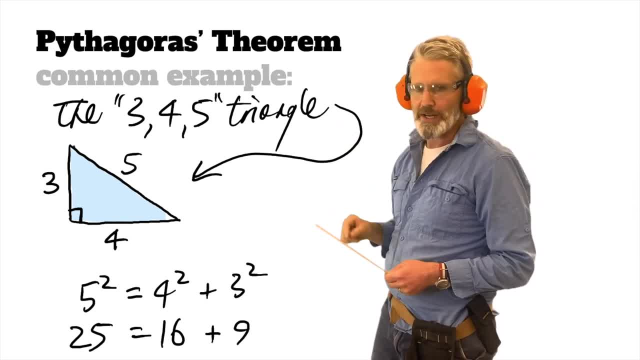 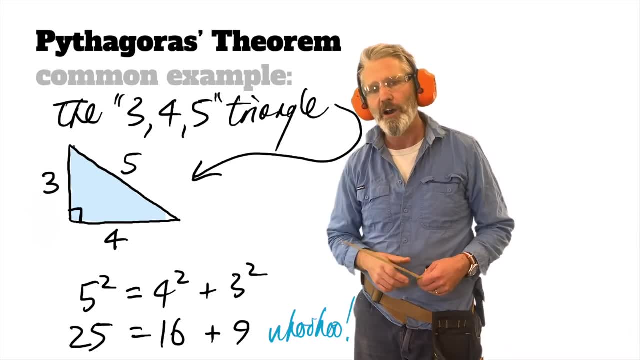 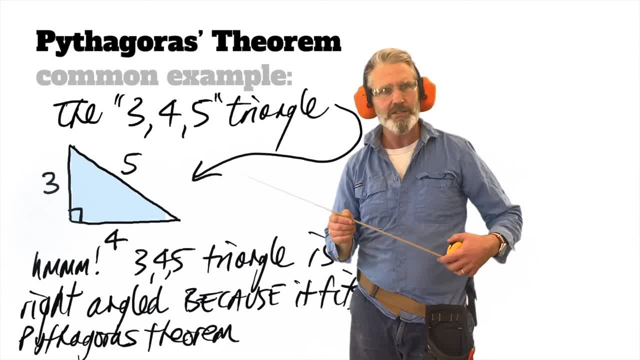 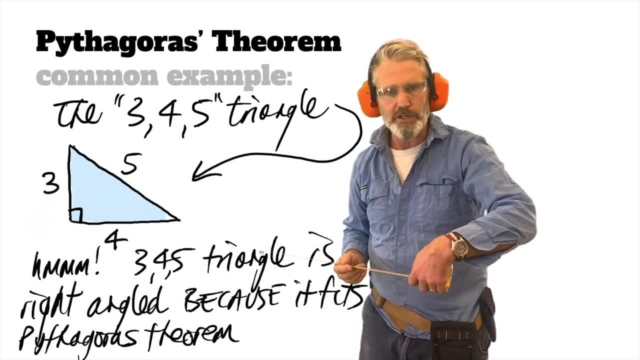 So, in other words, if we go and measure 3 metres along one side, 4 metres along another side, and if we made the diagonal or the hypotenuse to be 5, then you would have this really big square triangle. that's 3 metres. 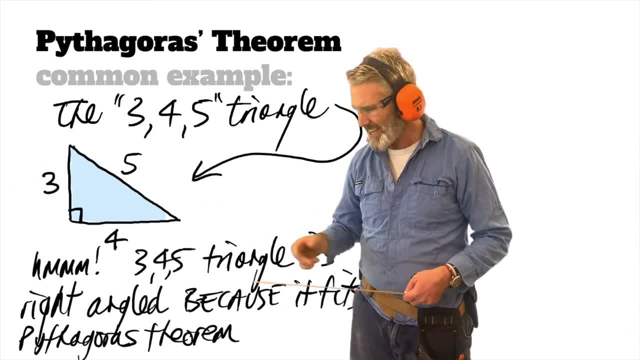 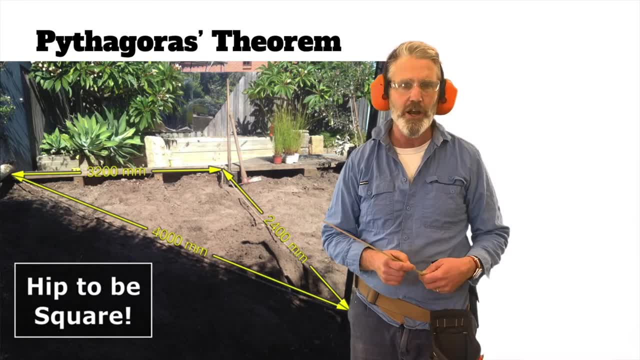 4 metres by 5 metres. Now, this set, this way of doing things, is used all the time for building to check things as square. The bigger the triangle that you can make all right, the more square you'll be, or the 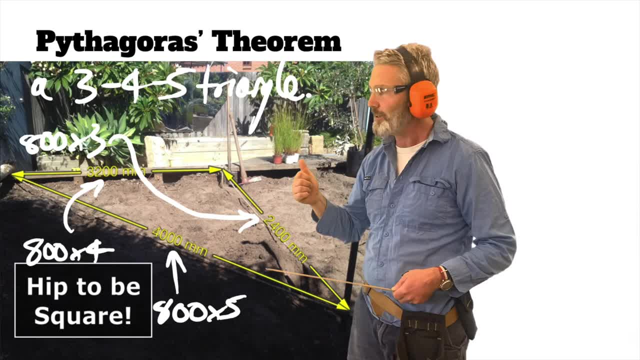 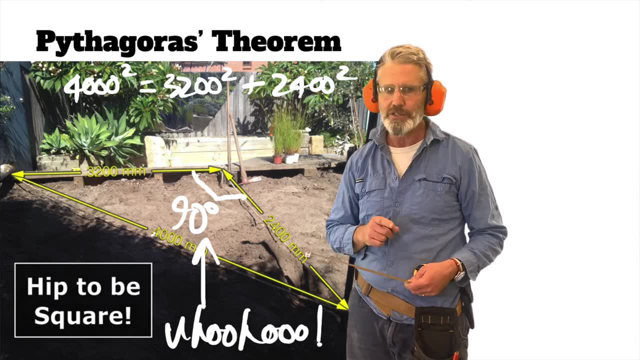 more accurate you'll be, So you can make it 30 metres by 40 metres by 50 metres, okay, or any combination of those. Now, 3-4-5 isn't the only ratio you can use, but anything with a hypotenuse squared equals. 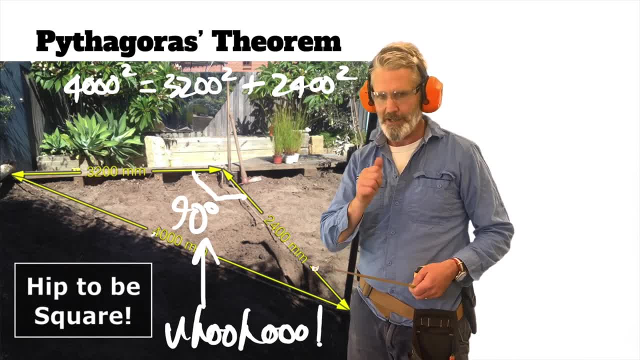 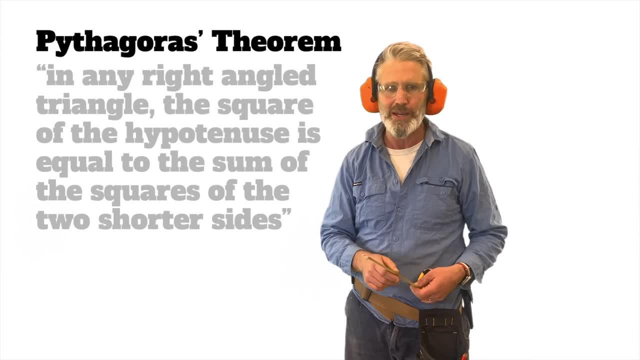 one shorter side squared Plus the other shorter side squared, and you're set. So welcome to the introduction of our Pythagoras Theorem. Yes, it is used for finding square and setting square, but it isn't used for finding how. 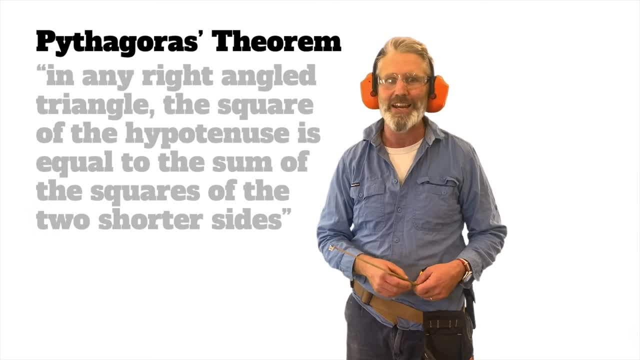 high a ladder leans up against a wall, So enjoy, Enjoy, getting some questions Woo-hoo.